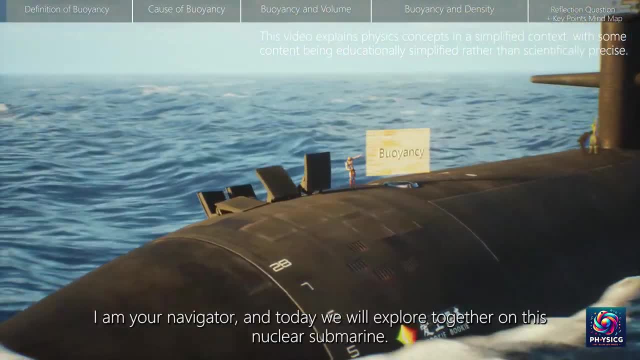 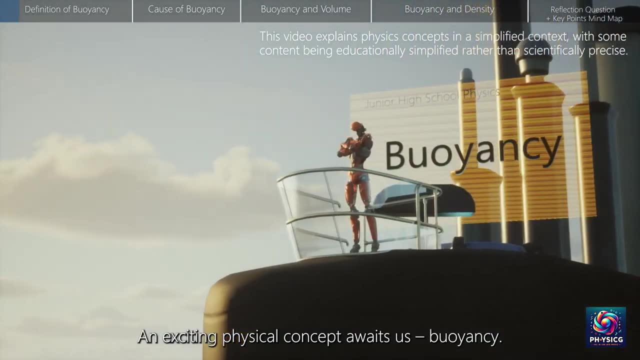 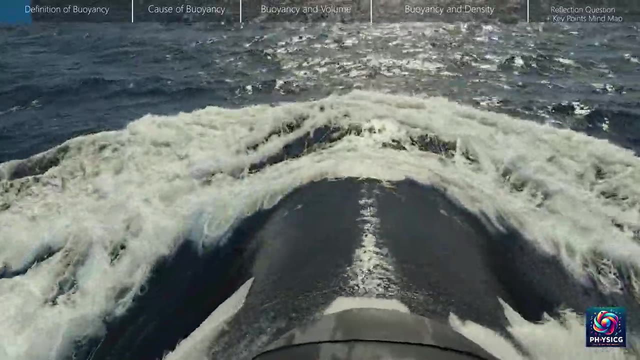 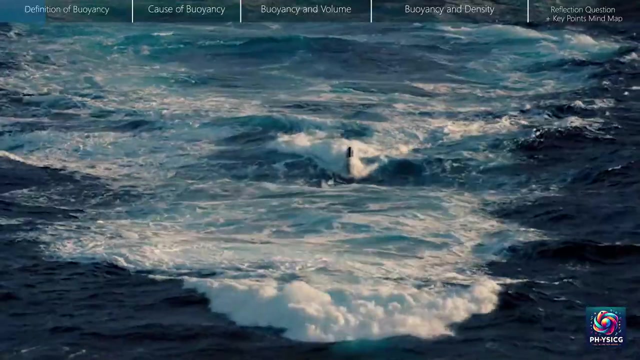 Welcome, students, to this mysterious ocean. I am your navigator and today we will explore together on this nuclear submarine. An exciting physical concept awaits us: buoyancy, Are you ready? Our adventure is about to begin. This profound ocean hides an unparalleled force. 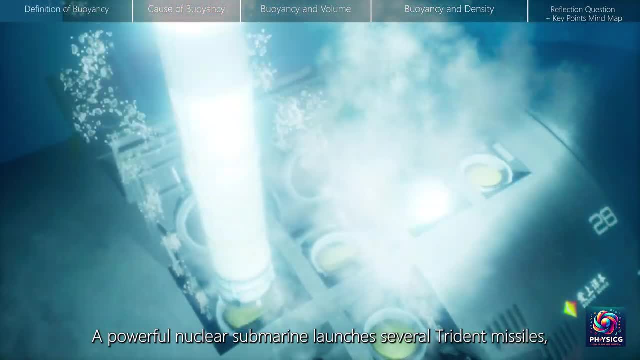 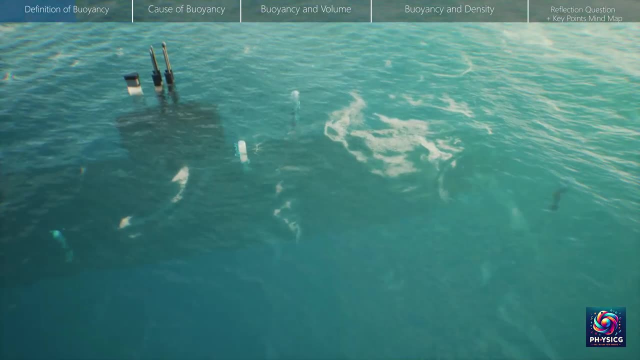 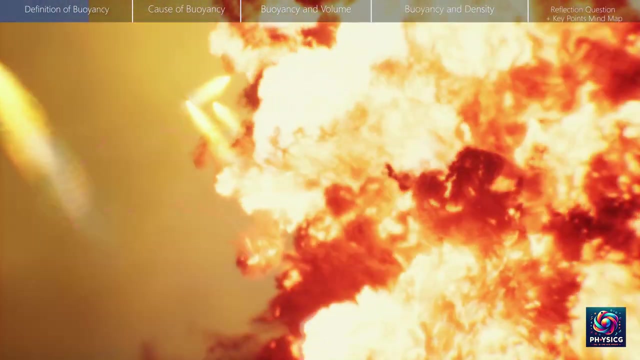 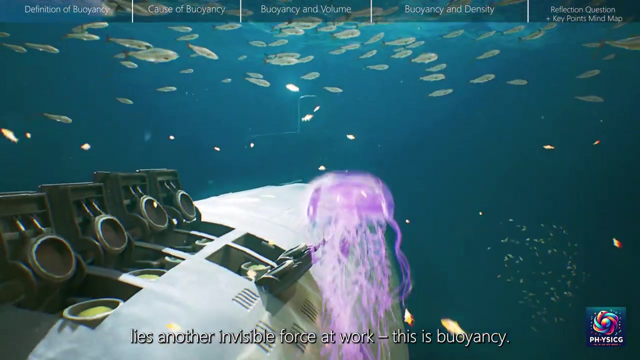 Right before our eyes, a powerful nuclear submarine launches several Triton missiles, breaking free from the water and soaring into the sky. However, behind this force lies another invisible force at work. This is buoyancy: Every object immersed in a gas or liquid. 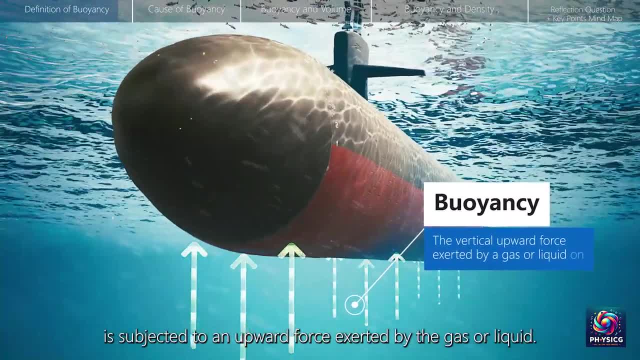 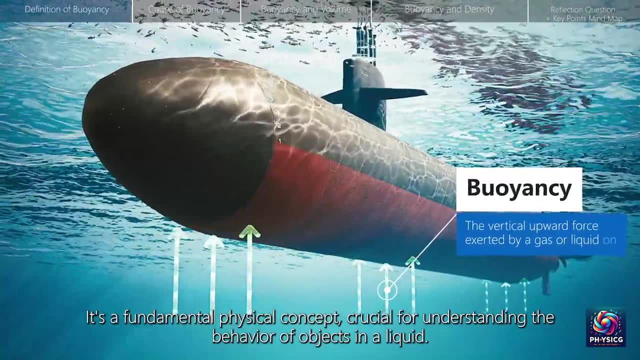 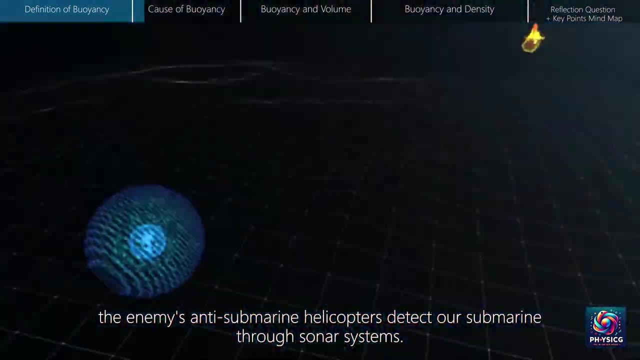 is subjected to an upward force exerted by the gas or liquid. This is buoyancy. It's a fundamental physical concept, crucial for understanding the behavior of objects in a liquid. As the nemesis of submarines, the enemy's anti-submarine helicopters detect our 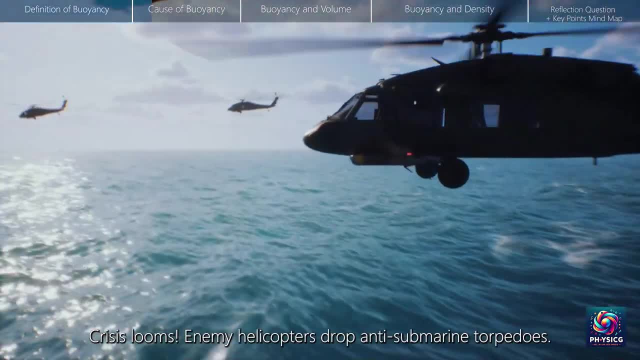 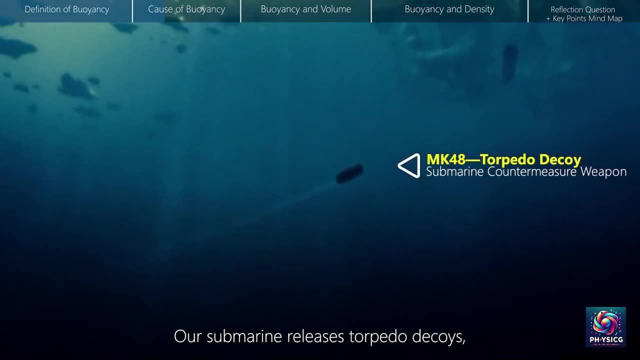 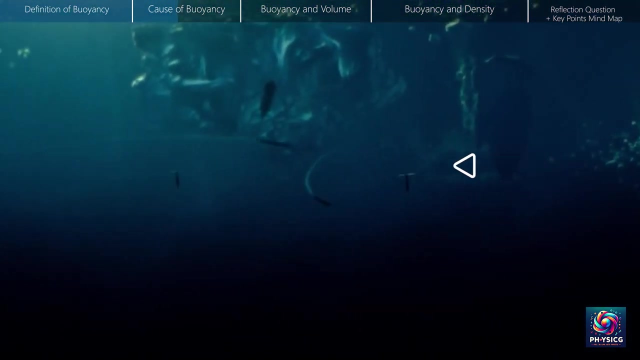 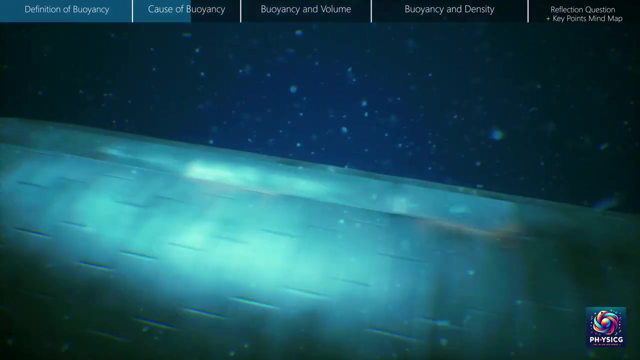 submarine through sonar systems. Crisis looms. Enemy helicopters drop anti-submarine torpedoes. Our submarine releases torpedo decoys, causing their torpedoes to lose their target. The submarine immediately reacts, beginning to dive into deeper, safer waters. 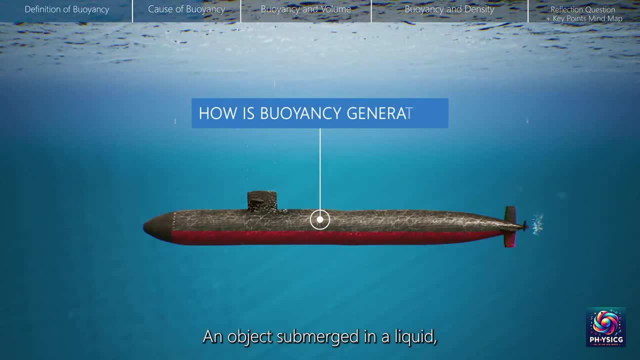 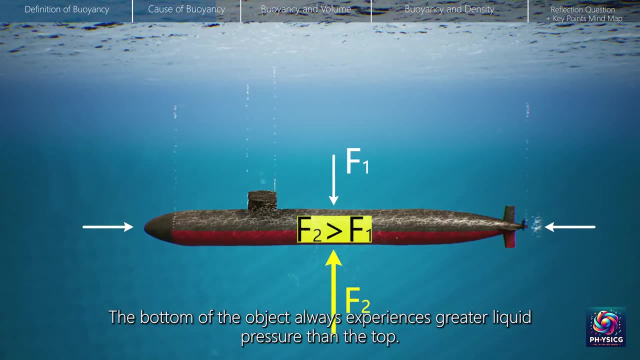 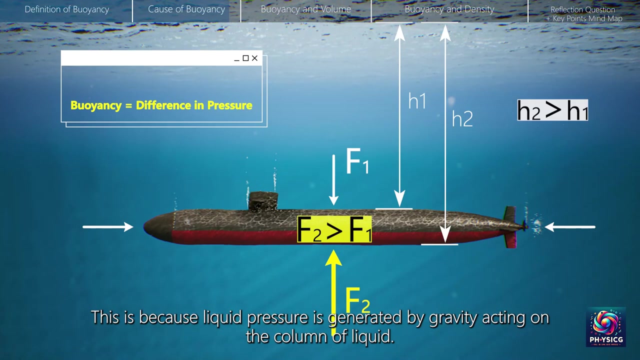 So how is buoyancy created? An object submerged in a liquid, like this submarine, experiences different pressures on its upper and lower surfaces. The bottom of the object always experiences greater liquid pressure than the bottom, the top. This is because liquid pressure is generated by gravity acting on the column. 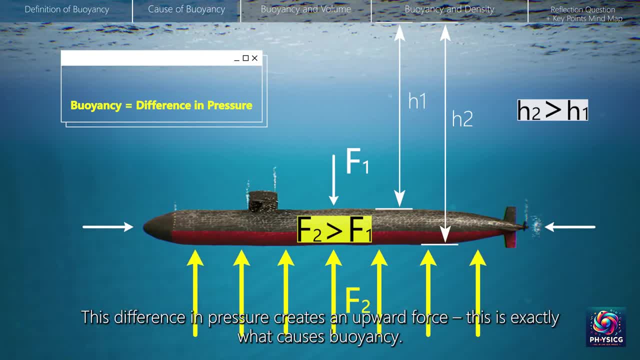 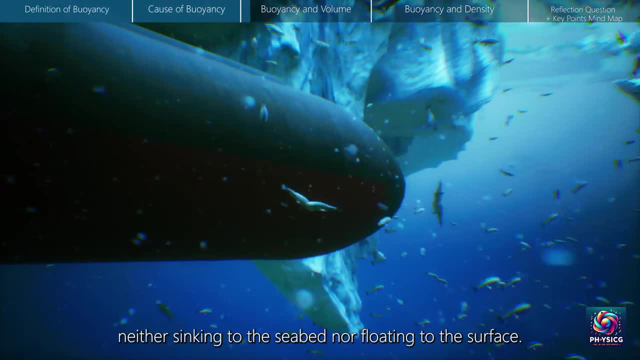 of liquid. This difference in pressure creates an upward force. This is exactly what causes buoyancy. Buoyancy allows the submarine to remain stable in the water, neither sinking to the seabed nor floating to the surface. After avoiding the crisis, the submarine proceeds. 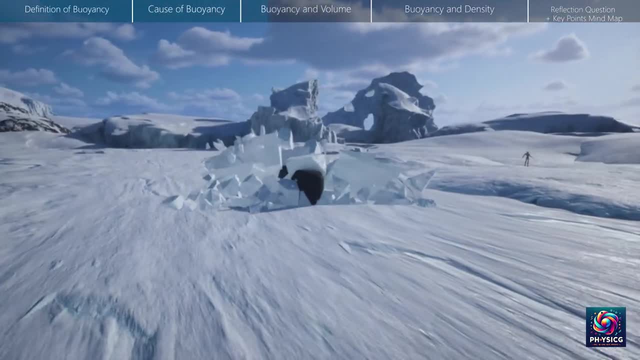 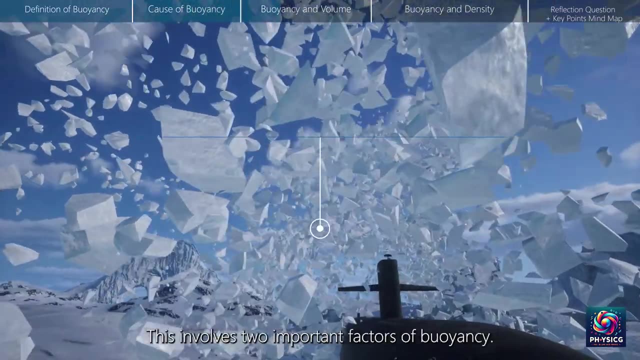 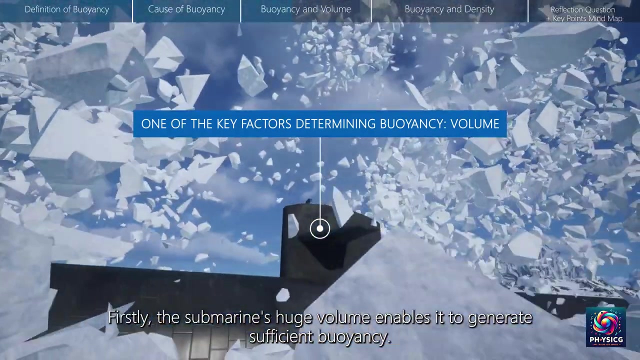 to its next mission. Its astonishing buoyancy enables it to easily break through ice. What is the source of this ability? This involves two important factors of buoyancy. Firstly, the submarine's huge volume enables it to generate sufficient buoyancy. This precisely. 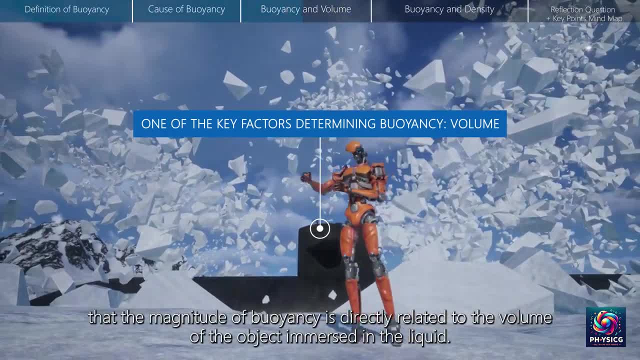 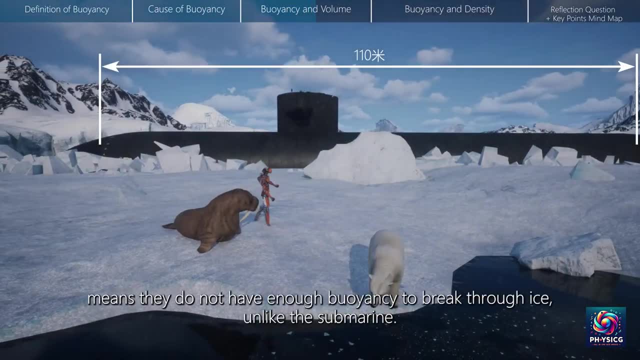 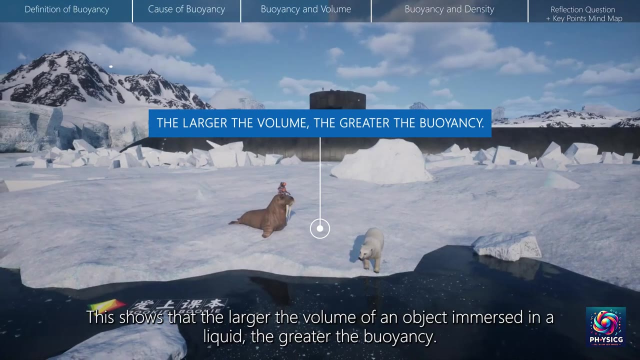 illustrates that the magnitude of buoyancy is directly related to the volume of the object immersed in the liquid. Look at these marine animals. Their smaller size means they do not have enough buoyancy to break through ice, unlike the submarine. This shows that the larger the volume of an object immersed in a liquid, the greater the buoyancy. 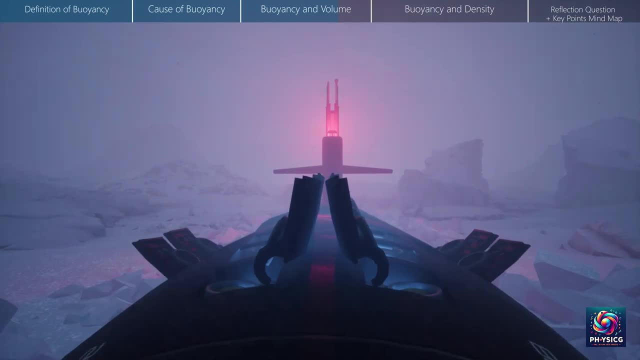 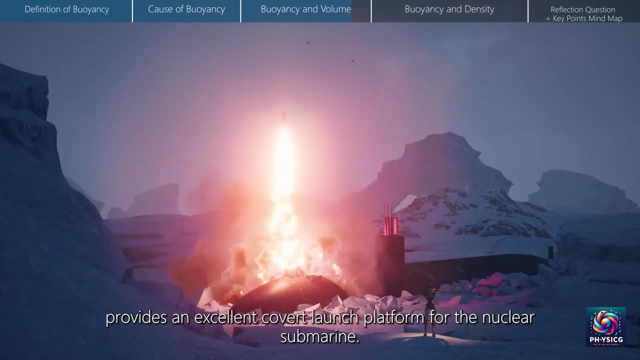 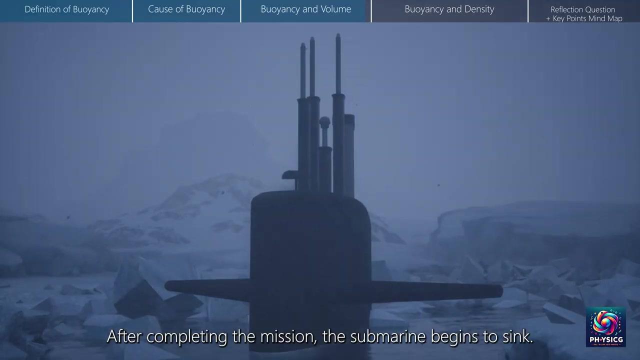 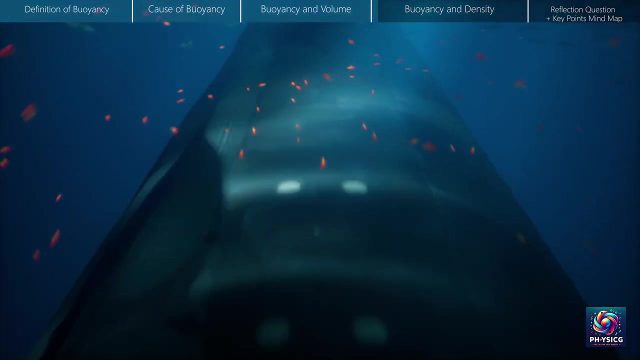 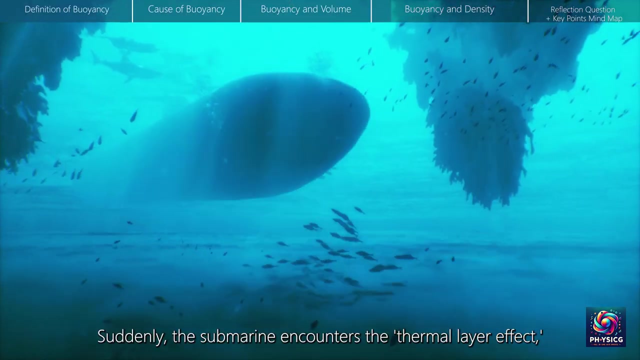 The remote and secluded Arctic region provides an excellent covert launch platform for the nuclear submarine. One launch can reach any target on Earth. After completing the mission, the submarine begins to sink. Suddenly, the submarine encounters the thermal layer effect, transitioning from a heavy water. 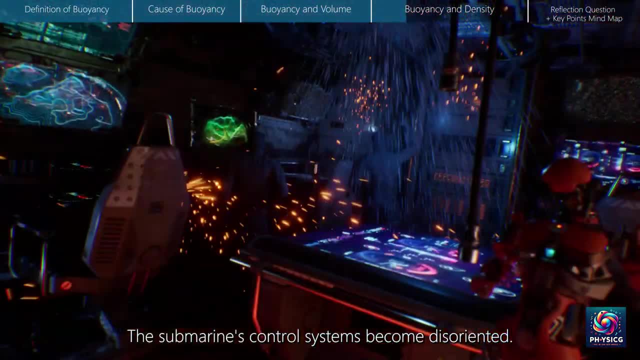 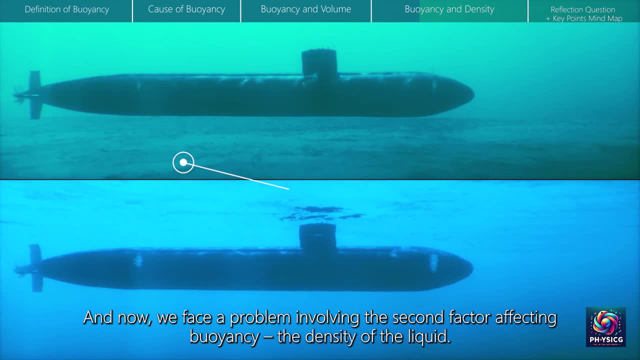 layer to a lighter one, The submarine's control systems become disoriented. We just discussed the relationship between buoyancy and the volume of an object, And now we face a problem involving the second factor affecting buoyancy: the density of the liquid, The high density. 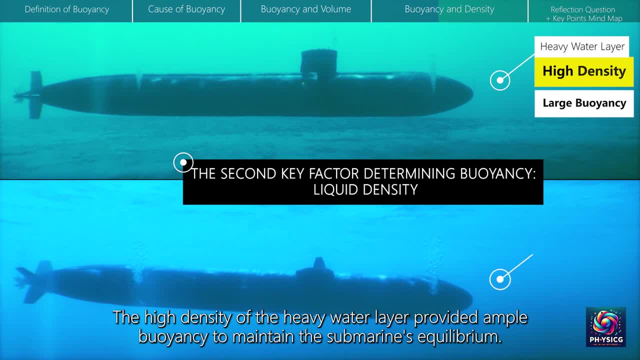 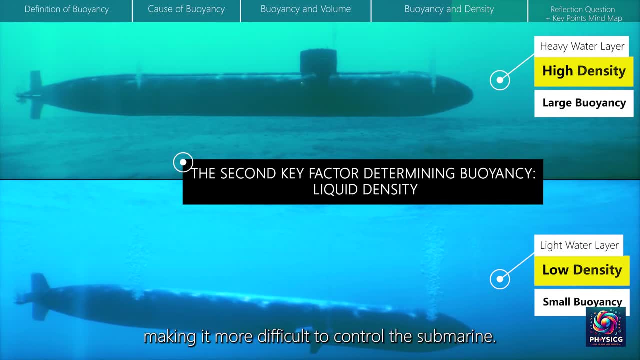 of the heavy water layer provided ample buoyancy to maintain the submarine's equilibrium, But in the lighter water layer the buoyancy is less than the buoyancy of the submarine. The lower the layer, the reduced density leads to decreased buoyancy, making it more difficult. 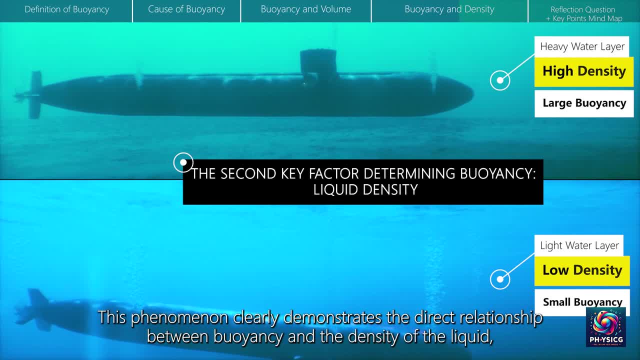 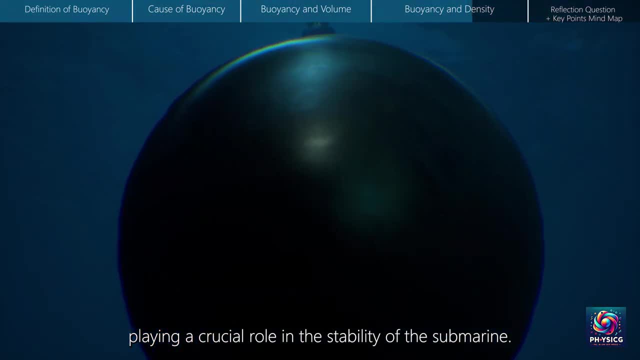 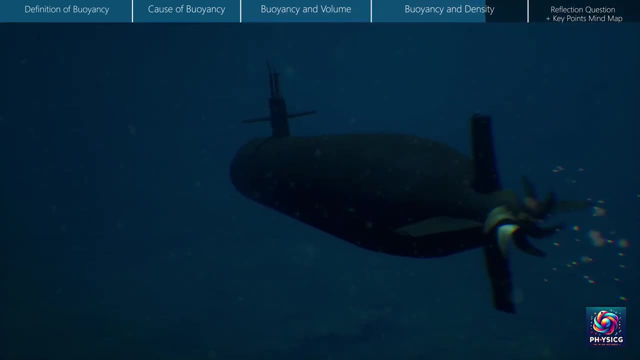 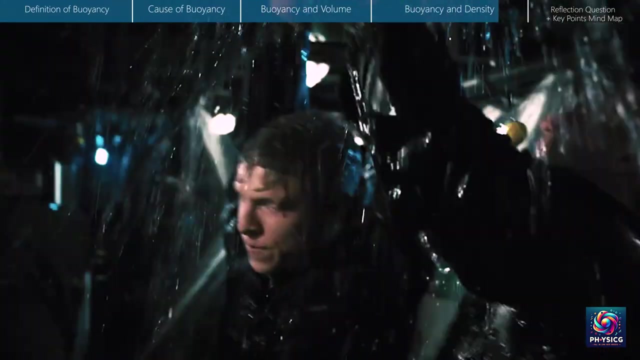 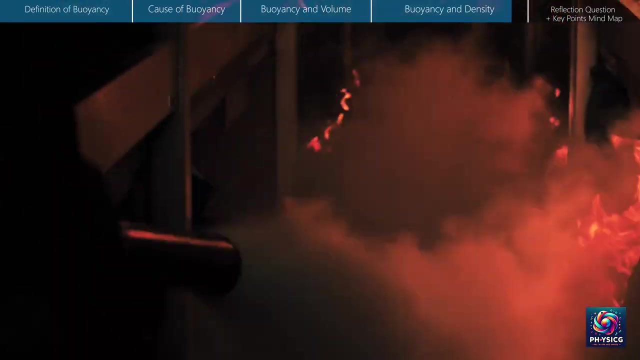 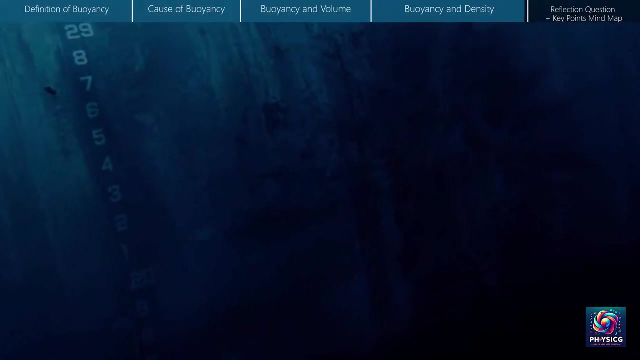 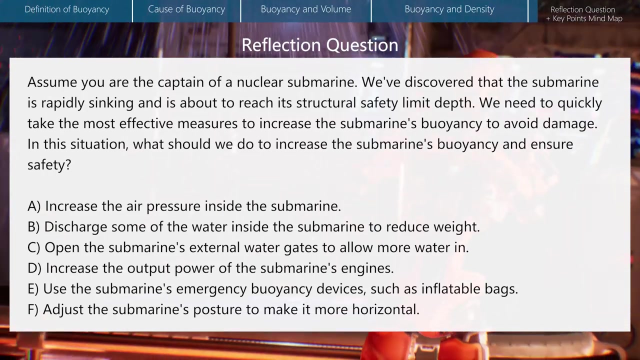 to control the submarine. This phenomenon clearly demonstrates the direct relationship between buoyancy and the density of the liquid, playing a crucial role in the stability of the submarine. Students, we are now facing an emergency situation. Assume you are the captain of a nuclear submarine. We've discovered that the submarine is rapidly sinking and is about 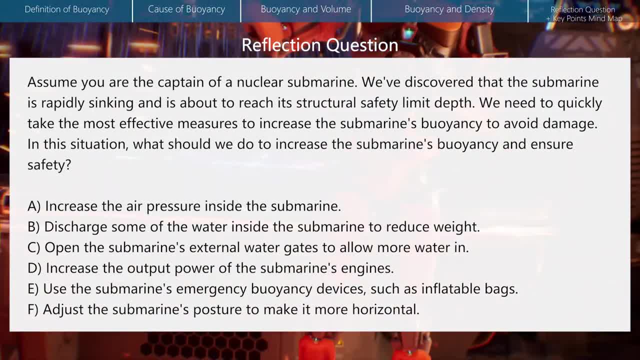 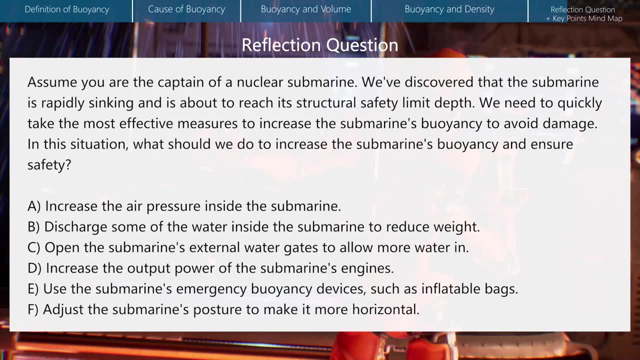 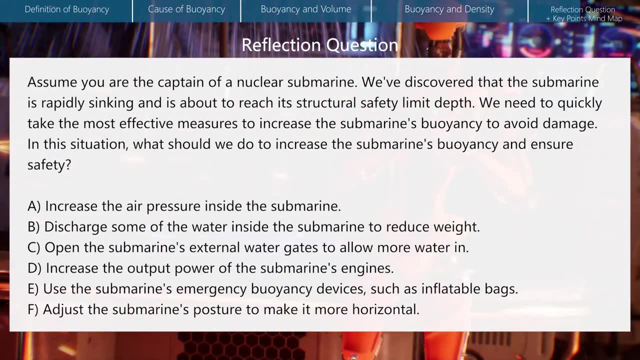 to reach its structural safety limit depth, We need to quickly take the most effective measures to increase the submarine's buoyancy to avoid damage. In this situation, what should we do to increase the submarine's buoyancy and ensure safety? A. Increase the air pressure inside the submarine.